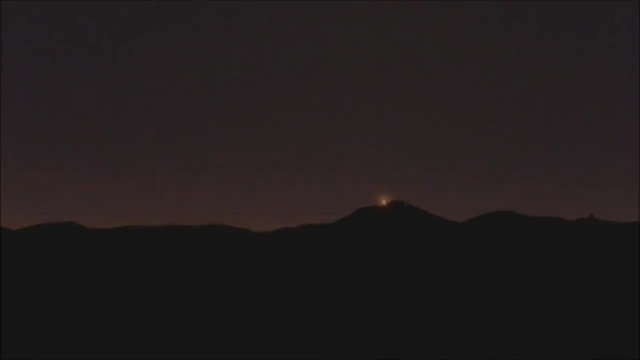 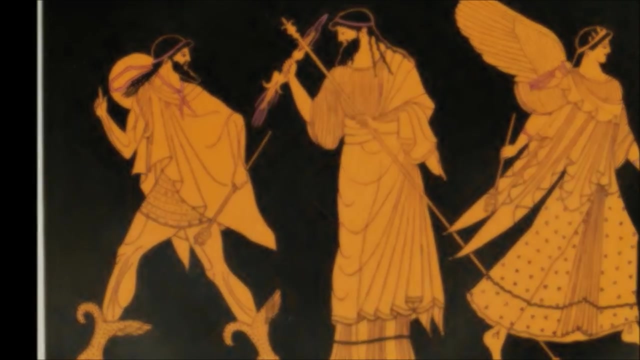 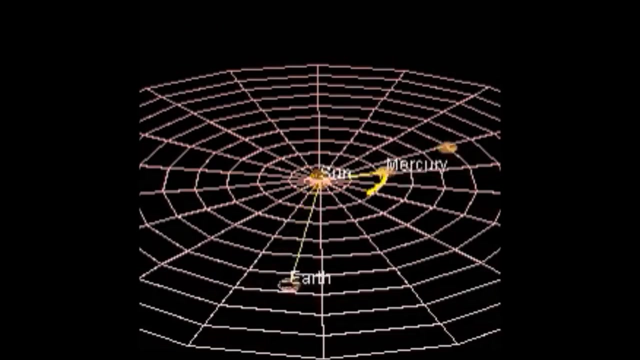 However, when Mercury can be seen, it shines brightly. Mercury was named for the Roman messenger of the gods, often shown wearing winged sandals, because of his great speed. Like the Roman Mercury, the planet Mercury is very fast. It has the shortest orbit of any planet in the solar system, completing an orbit around. 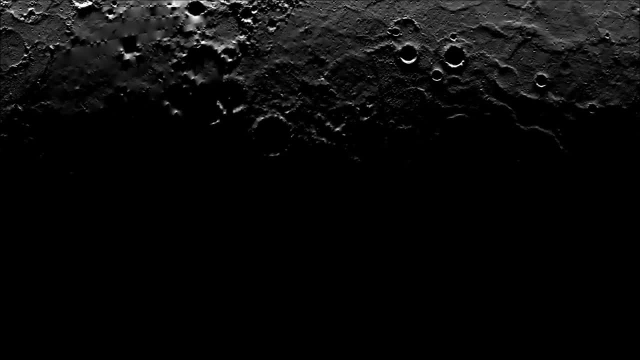 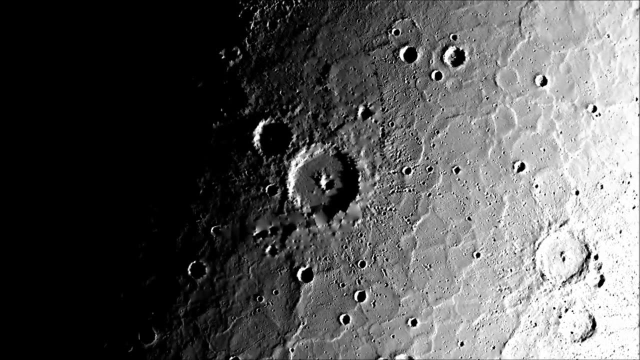 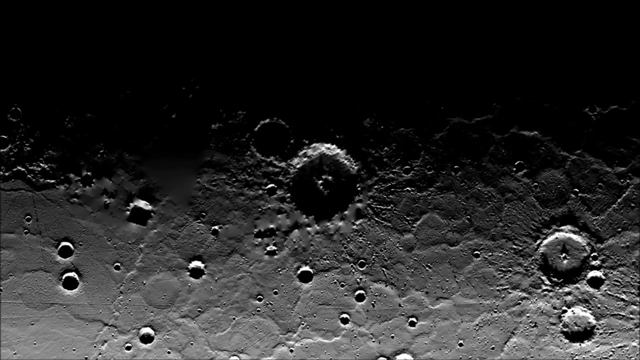 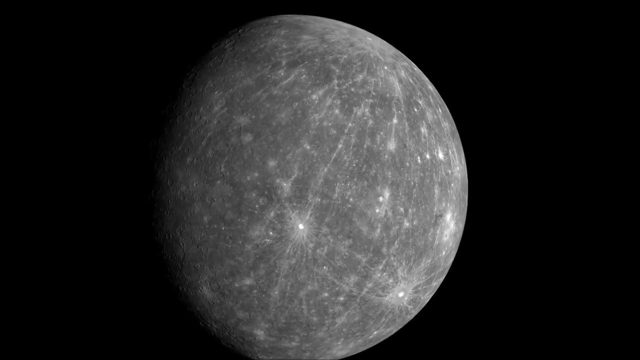 the sun in just 88 days. Although Mercury orbits the sun much more quickly than the Earth, it takes much longer for it to rotate. Earth rotates once every 24 hours, but Mercury only rotates once every 59 days. Although it is the closest planet to the sun, Mercury is not the hottest. 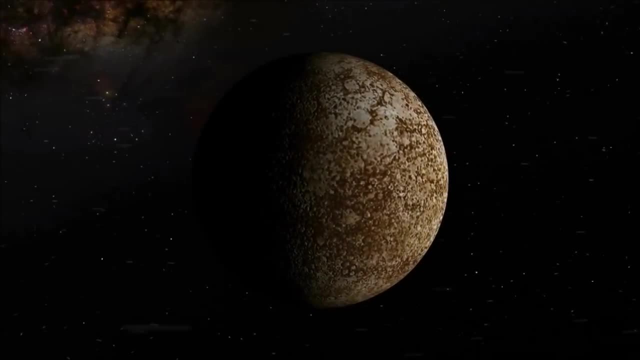 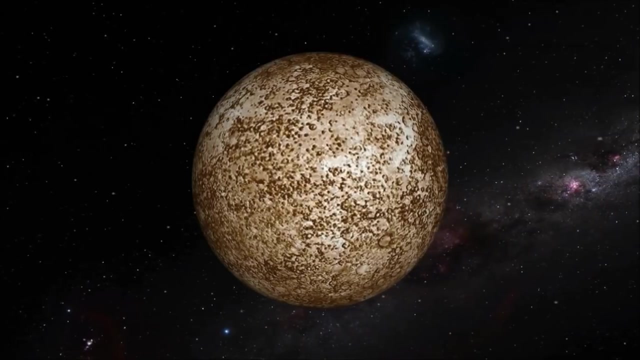 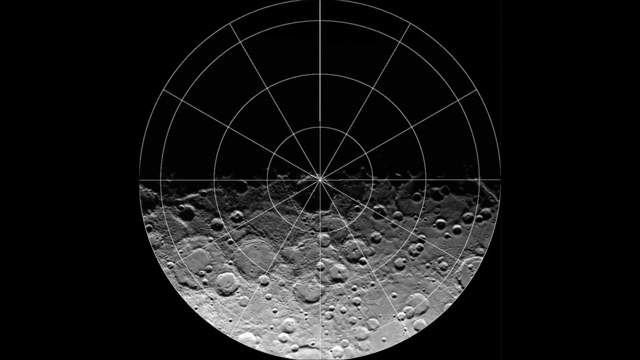 Because it has almost no atmosphere. the heat that comes to it from the sun quickly escapes back into space. Still, the environment on Mercury is harsh. Thanks for watching. In the sunlight, temperatures reach hundreds of degrees. At night, temperatures fall far below freezing. 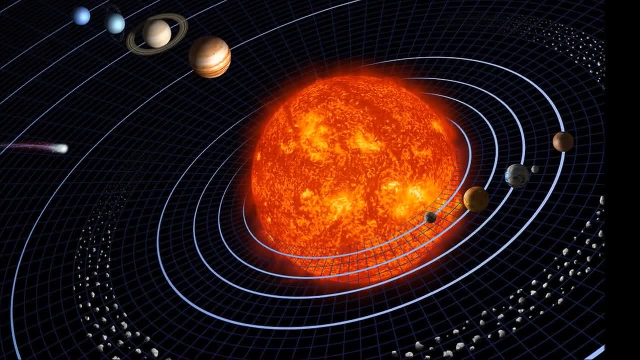 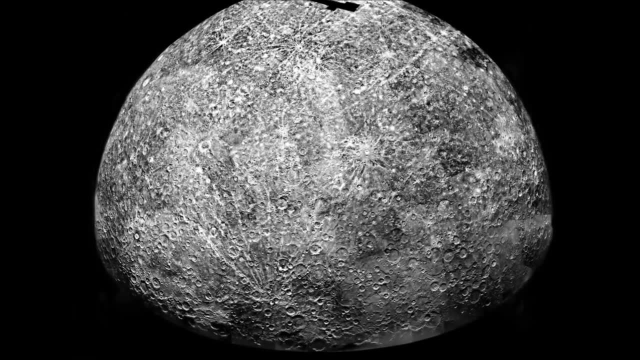 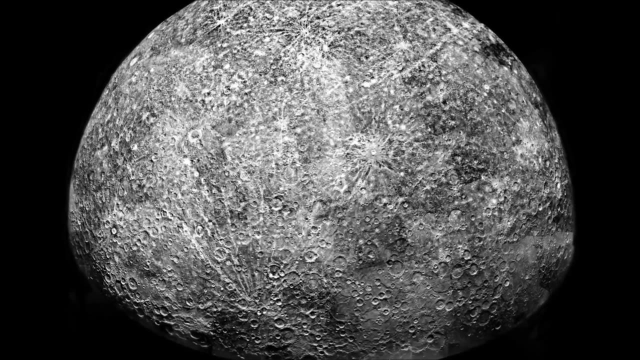 One of the four inner planets in the solar system. Mercury has a rocky body like the Earth. Mercury's surface is solid and covered with craters. It has no moons of its own and it has no rings. In appearance, Mercury closely resembles our Moon. 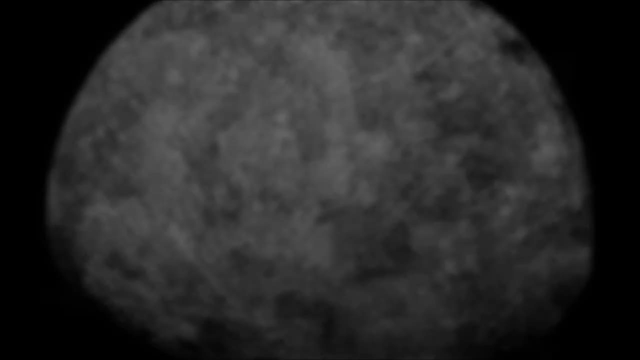 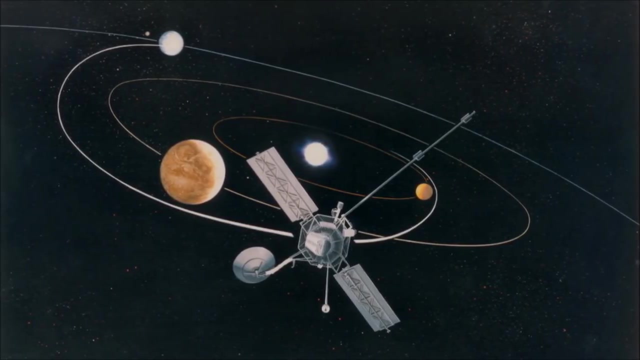 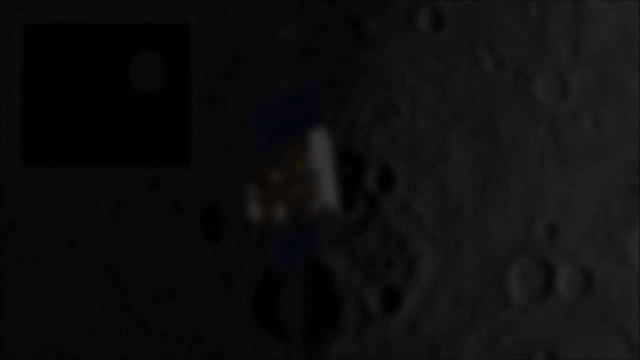 Two spacecraft have visited Mercury. In 1975, Mariner 10 provided the first up-close images of Mercury's surface, mapping about 45 percent. In 2011,, the MESSENGER mission achieved an orbit around Mercury which has allowed much. 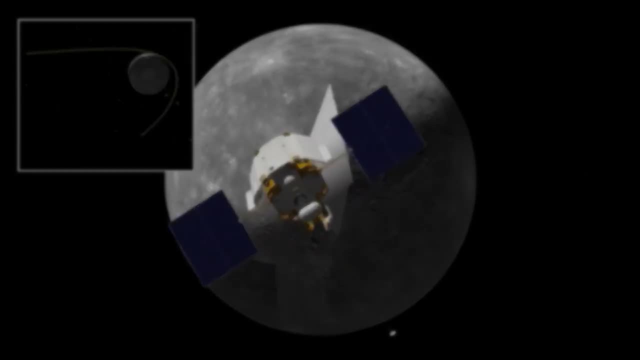 of the remaining surface to be mapped, Although its surface is quiet now. the MESSENGER spacecraft have been Florenc E coli, Okinawa and Par�íi, the Black Sea, for more than a decade In anti-Earth climate conditions. Mercury has become a surprisingly resilient planet. Mercury's surface is solid and its surface is calmer than most other planets. Mercury's surface is solid and its surface is calmer than most other planets. In appearance, Mercury has a disappeared surface. Mercury has a disappeared surface. In appearance, Mercury has a disappeared surface. 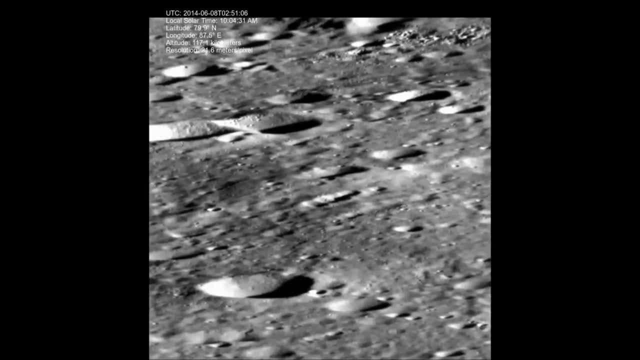 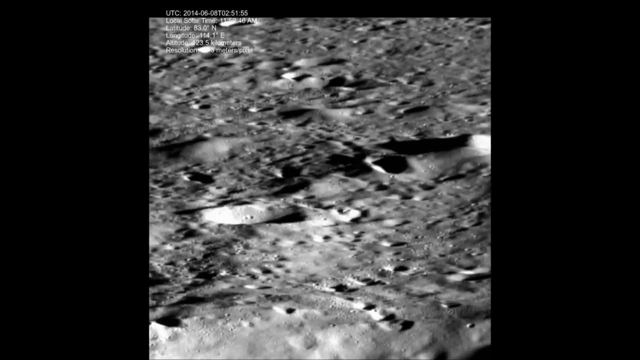 In appearance. Mercury has a disappeared surface. Mercury has a disappeared surface. spacecraft discovered evidence that Mercury once had active volcanoes on its surface. Shield volcanoes and ancient lava flows were revealed in the images that MESSENGER relayed to Earth.